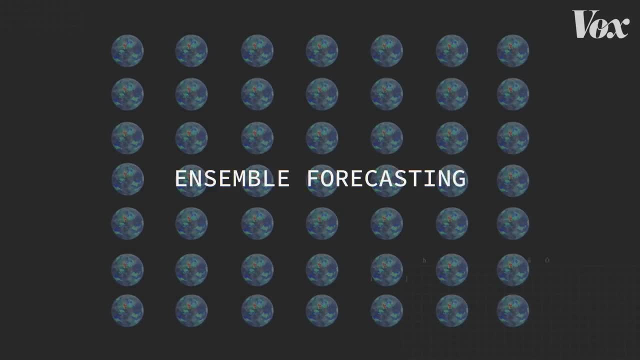 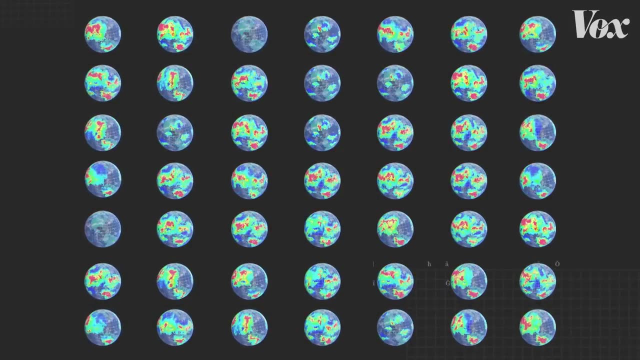 It's called ensemble forecasting and it helps meteorologists measure uncertainty. If all 50 forecasts look similar, there's a higher certainty in the prediction, But if there's a lot of variation, there's much less. We've got to kind of keep an eye to the sky. 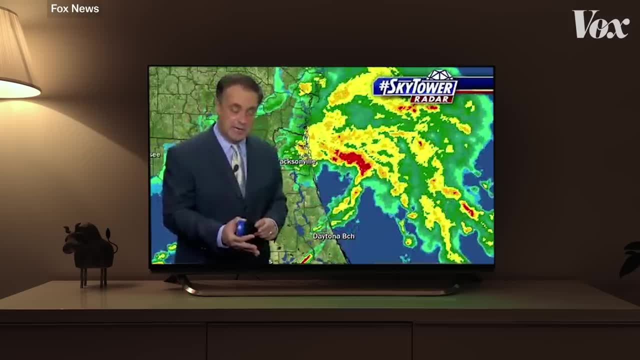 There's a potential of another storm in the works. This went from zero percent chance to 40 percent at 2 o'clock, 70 percent at 8 o'clock And at 11 o'clock we had a tropical storm. Weather centers only release their forecasts. 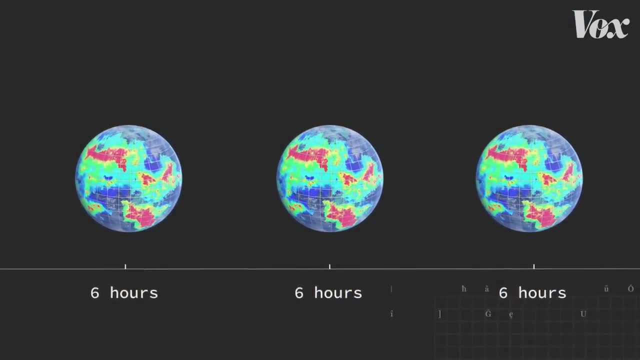 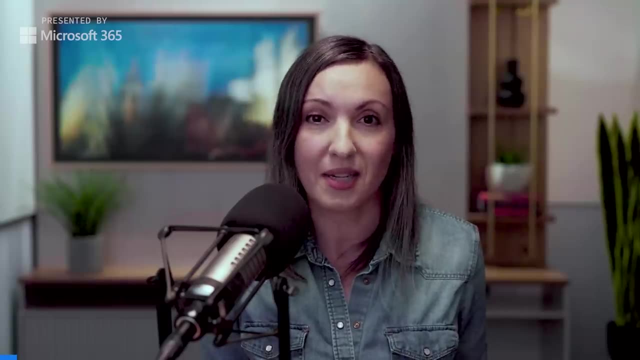 Every six hours, because that's all today's computing power will allow. But what if that limit didn't exist? Before we explain that, we'll hear from the sponsor of this video. This episode is presented by Microsoft Copilot for Microsoft 365, your AI assistant at work. 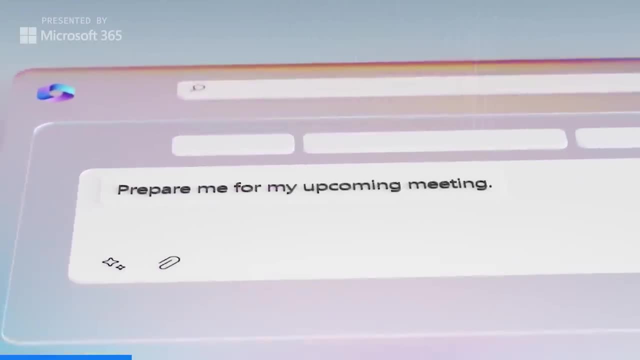 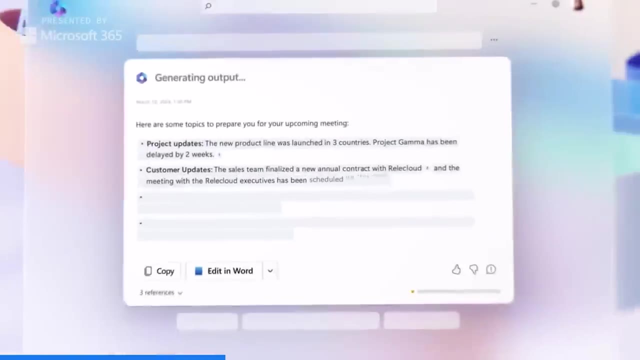 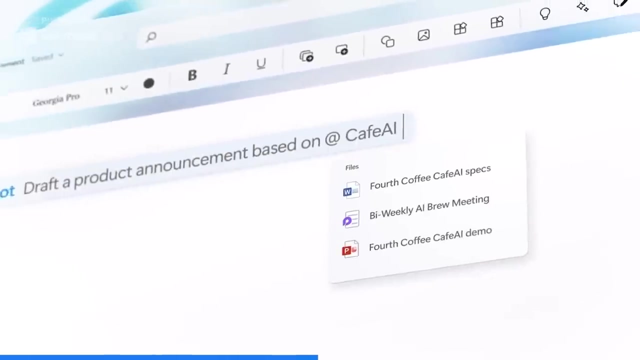 Copilot can help you solve your most complex problems at work, going far beyond simple questions and answers: From getting up to speed on a missed Teams meeting in seconds to helping you start a first draft faster in Word. Copilot for Microsoft 365 gives everyone an AI assistant at work in their most essential apps to unleash creativity, unlock productivity and up-level skills. 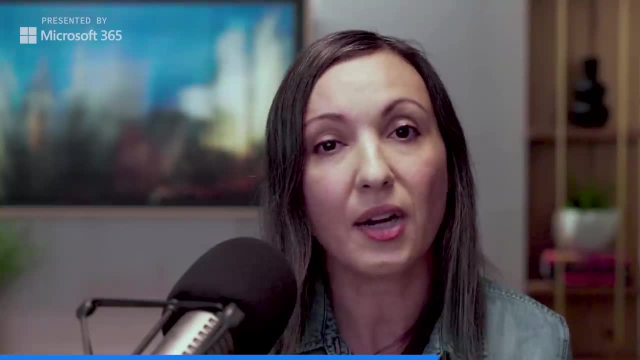 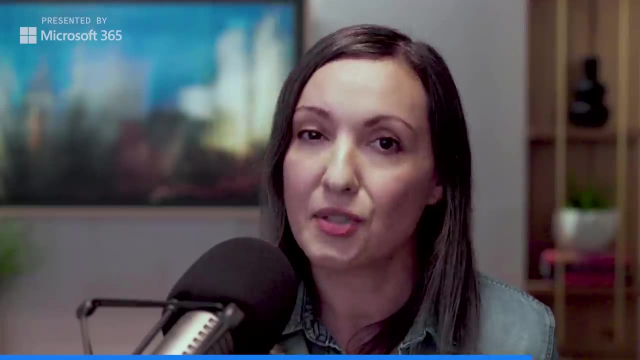 And it's all built on Microsoft's comprehensive approach to security, privacy, compliance and responsible AI. Microsoft does not influence the editorial process of our videos, but they do help make videos like this possible. To learn more, you can go to Microsoftcom slash Copilot for work. 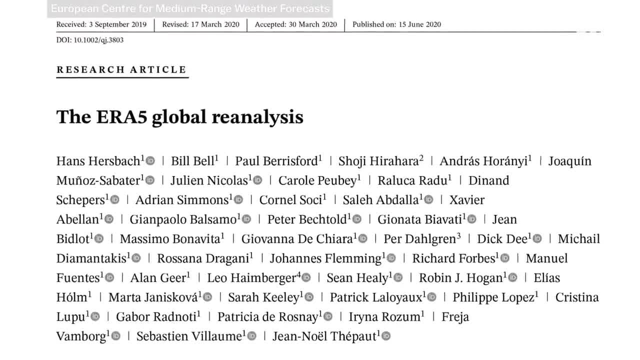 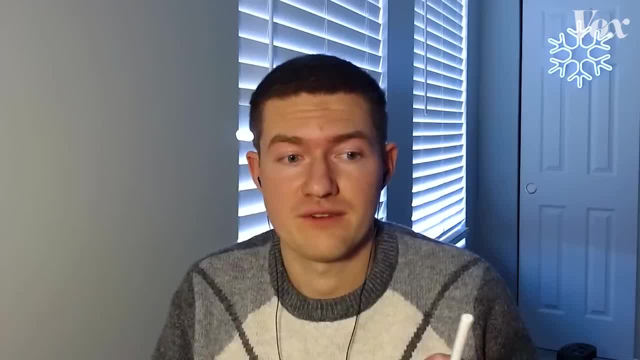 Now back to our video. In 2020, a group of researchers published a data set called ERA-5, which contained about 40 years of the Earth's hourly weather data. That data set was just primed for using AI because it was huge. 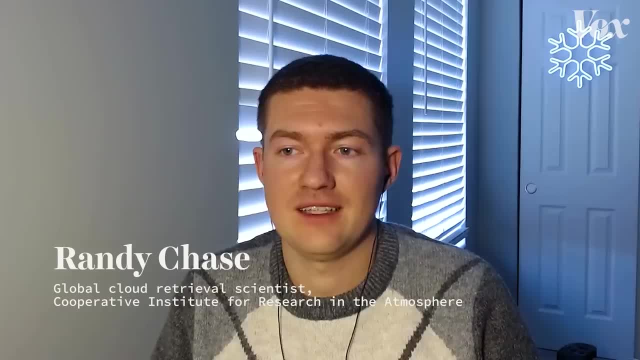 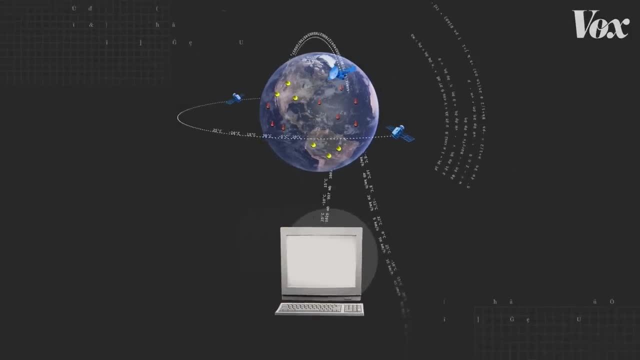 The data is nice and smooth, There's no missing values And it's free just to step in and say, hey, you have terabytes of data. I can learn how weather moves. AI models learned how weather moves, not through applying trillions of physics equations to the Earth's atmosphere. 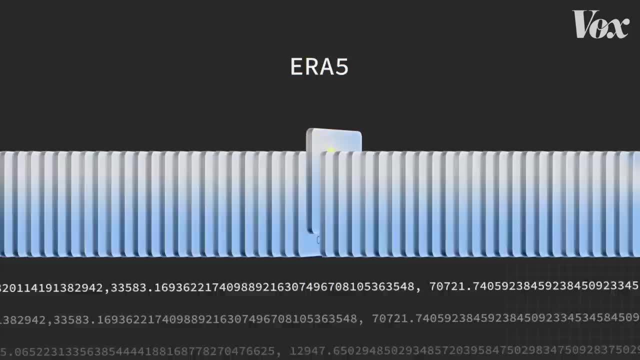 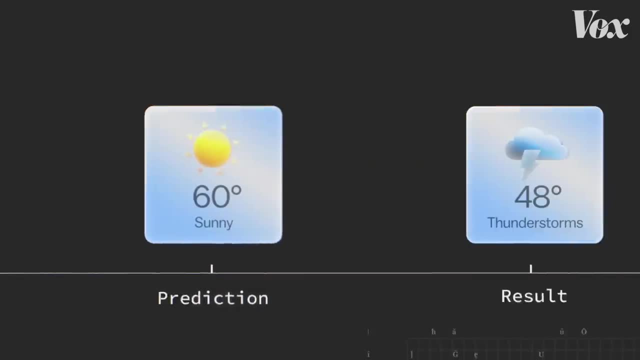 but by being trained on ERA-5's enormous historical data set. Researchers gave the models a snapshot of weather conditions, asked them to make a prediction and then scored them on how closely that prediction matched what really happened. After a while, the models eventually got really good at this. 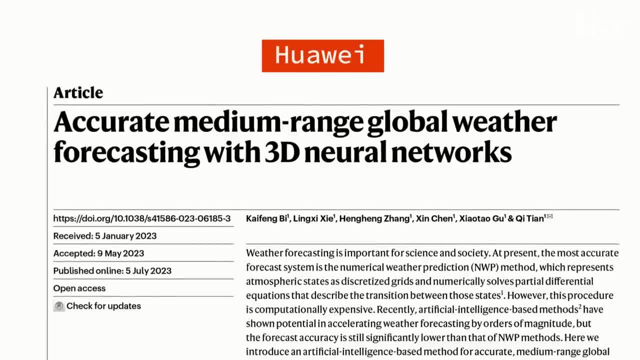 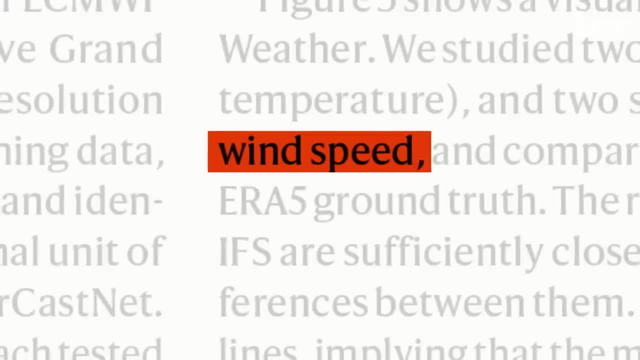 By 2023, the tech companies Google, Huawei and NVIDIA had developed models that rivaled traditional forecasting on variables like surface temperature, humidity and wind speed, and on some extreme weather events, like the paths of tropical cyclones, atmospheric rivers and extreme temperatures. 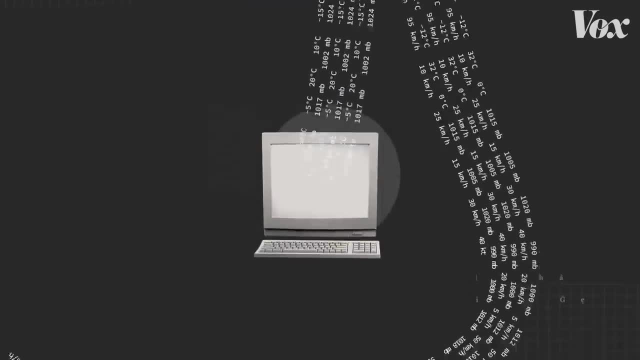 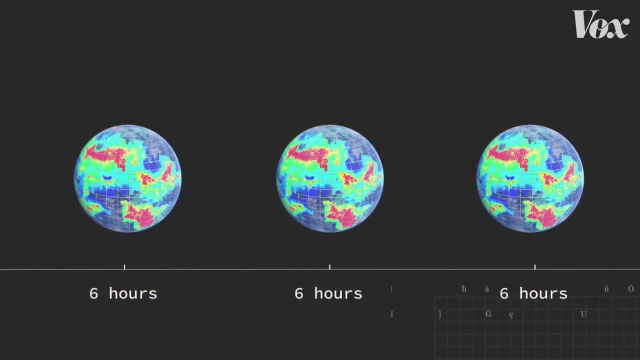 These AI models still exist. They still rely on the same observation data from the big weather centers- the data that creates that initial 3D grid snapshot- But they don't require anything close to six hours to produce a prediction. Huawei's Pengu weather model, for example, can produce a week-long forecast in 1.4 seconds. 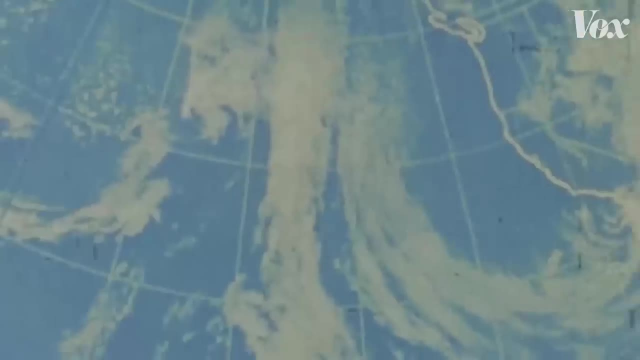 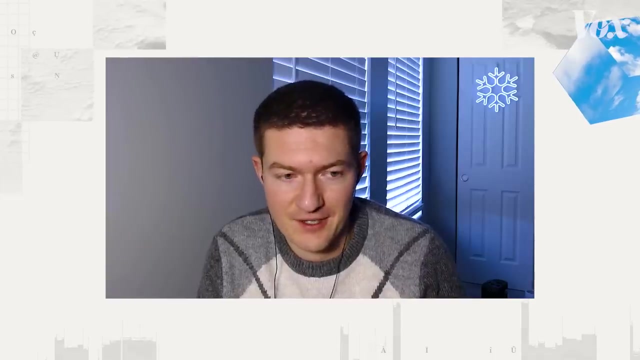 which means that we spent over a century figuring out the physics, the atmospheric science and the computational skill to bring us our modern-day weather forecast, And now, suddenly, we have these AI models that have come out of you know the past two, three years. 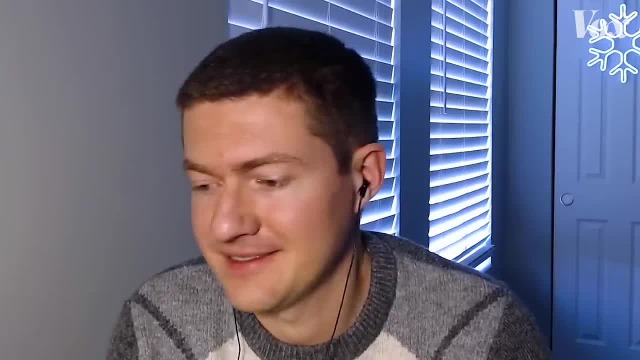 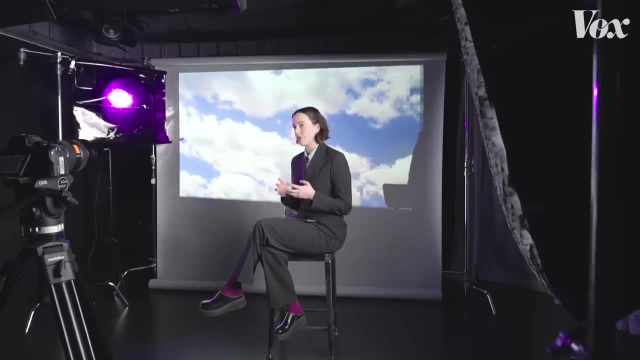 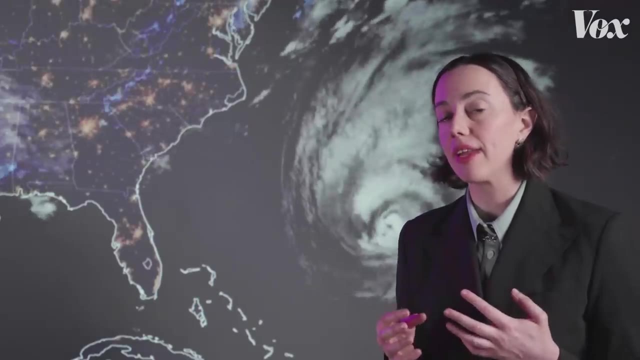 and they're getting the same skill, and now they run on a modest laptop. Despite the impressive results from these first AI models, there's still lots of work to do. Google's GraphCast predicted Hurricane Lee's path faster than traditional models, But it didn't prove it could predict a hurricane's intensity, which is a trickier calculation to make. 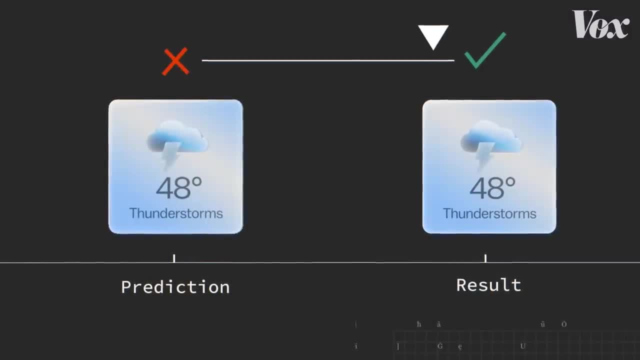 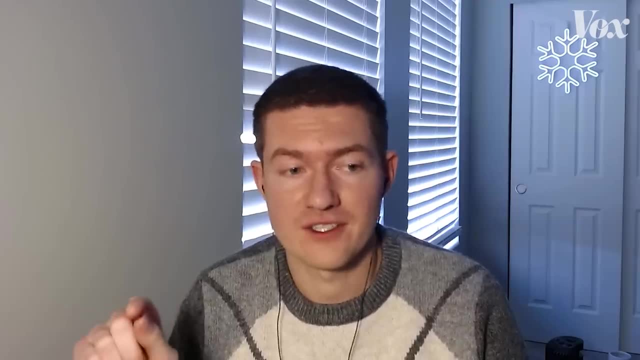 These AI models are incentivized to get as many correct answers as they can through the scoring system. If you swing for it, swing for the fences right. If it misses the model, The model is penalized very large. It says no. you should never do that. 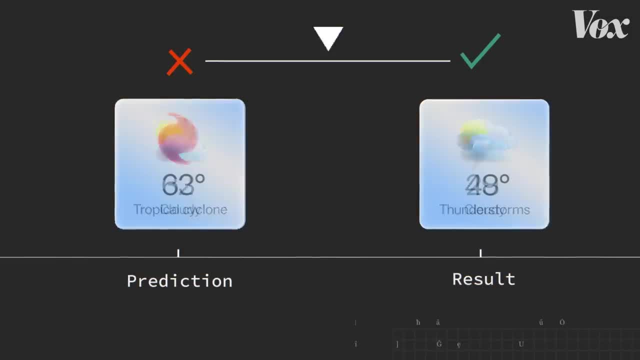 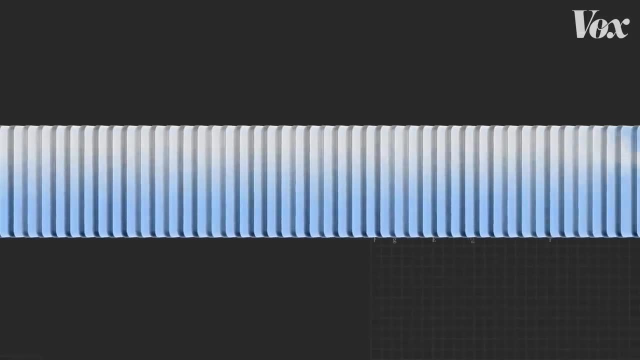 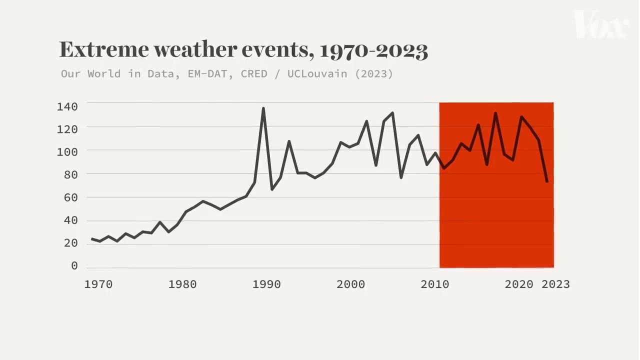 Don't swing for the fences because the error is going to be huge. But by prioritizing safer, correct answers to boost a model's score, it could miss rare, outlier weather events. Plus, they are learning from 40 years of history, And historical weather has fewer extreme events than we do today or will have in the future due to climate change. 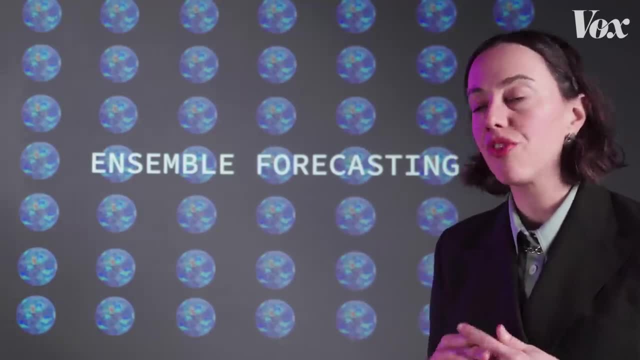 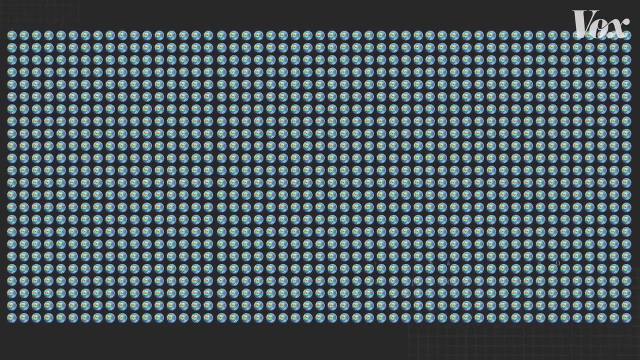 But a big reason for optimism with these AI models comes from their ensemble forecasting. Instead of the traditional 50 ensemble forecasts, they can predict a thousand or more because they're freed from computing and time constraints. There's always going to be uncertainty in a weather prediction. 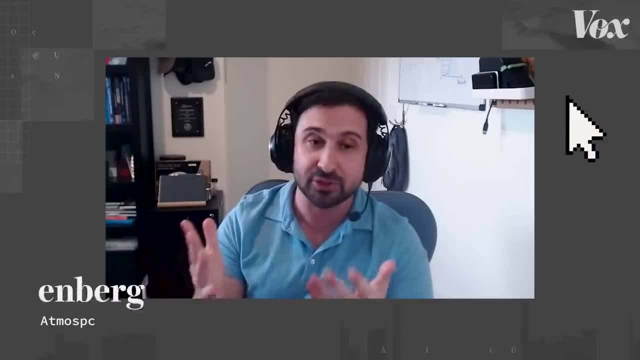 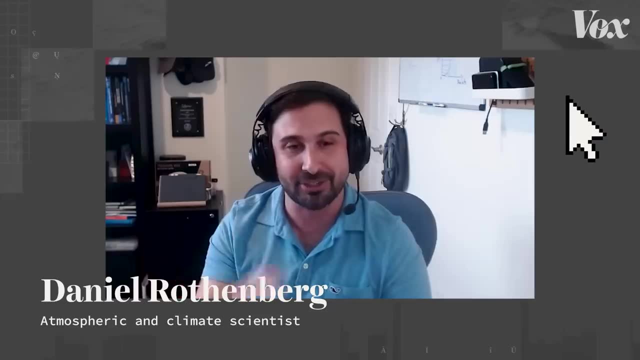 But larger ensembles will help us measure that uncertainty better. That's an extremely useful context to say: you are a emergency manager down in Florida who's dealing with a very difficult decision: Are you going to, you know, order an evacuation or not? 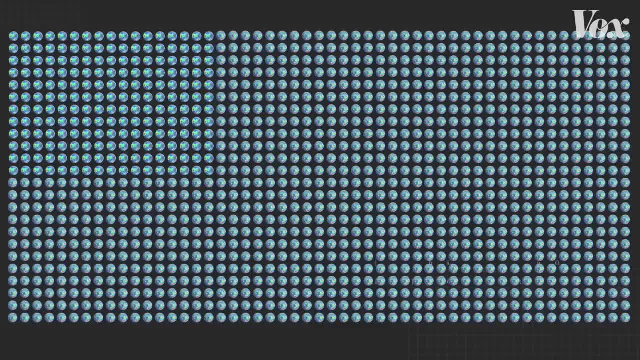 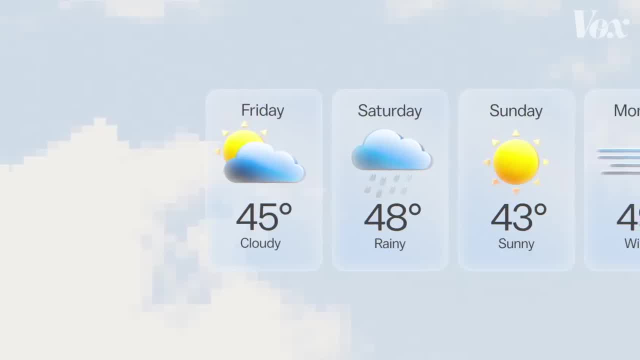 You want as much information about the uncertainty as possible. Large ensembles might also catch a rare weather event that a 50 member ensemble would miss or measure the probability that it will miss. Or measure the probability that it will miss. Or measure the probability that it will miss.